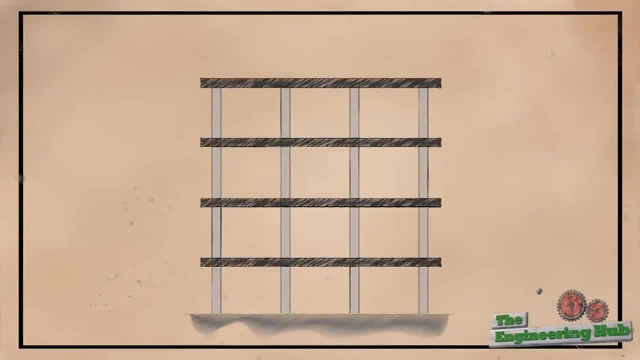 during its life. For their entire life, structures are subjected to gravity loads. Gravity loads consist of any mass that is accelerated by gravity and pushes vertically down on the structure. These masses can be the mass of the building material itself, accumulated snow or human actions. Engineers have become very good at 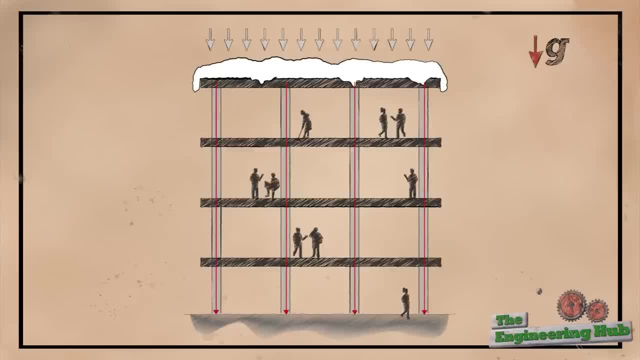 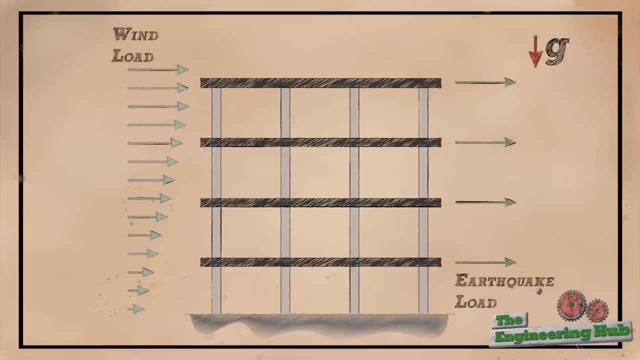 dealing with gravity loads. Most of the time, these loads are transferred to the ground with an outstanding success. Besides gravity loads, there are also lateral loads, which act in a horizontal direction. These loads are then transferred to the ground by gravity loads. 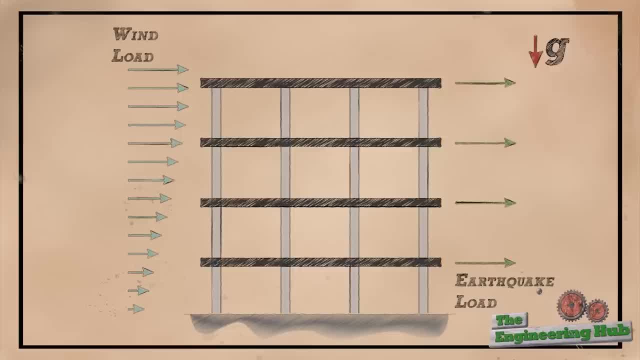 These loads are then transferred to the ground in a horizontal direction, such as wind or earthquake loads. The earthquake loads occur as a result of ground acceleration or shaking that is transferred to the building. This is pretty intuitive and can be replicated with a stack of blocks. 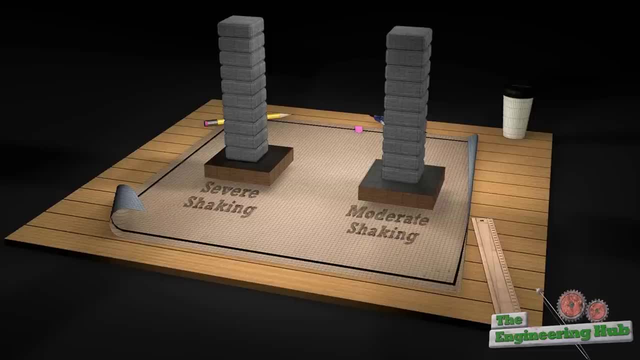 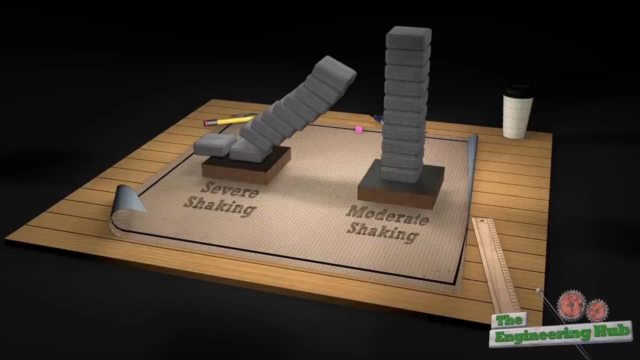 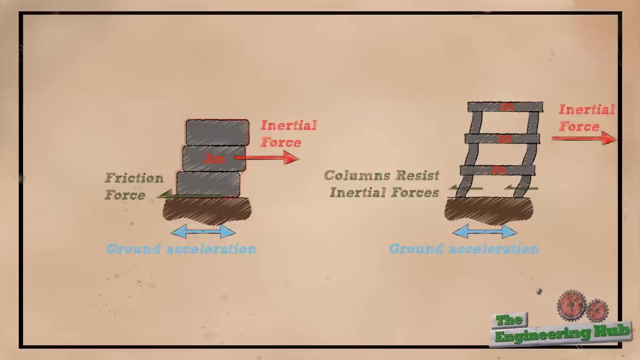 If the system is accelerated fast enough, like the stack on the left, the inertial forces of each block will overcome the frictional forces and separate from the stack. This analogy can be extended to structures, Although structures are flexible and do not displace rigidly, but rather deform internally. This internal deformation. 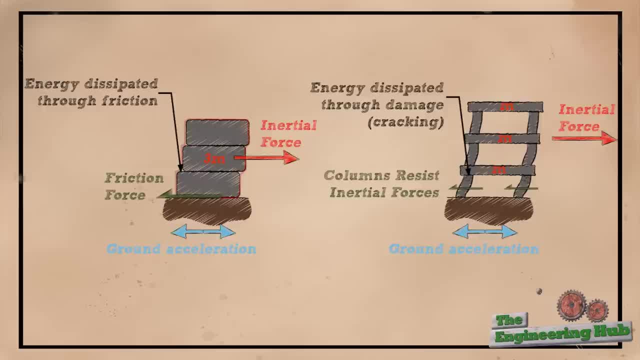 is shown in terms of sustained damage and is key in dissipating a portion of the kinetic energy transferred from the moving ground into the building. But the reason why damage occurs in the first place can be traced back to Newton's second law: Any accelerated mass requires that same. 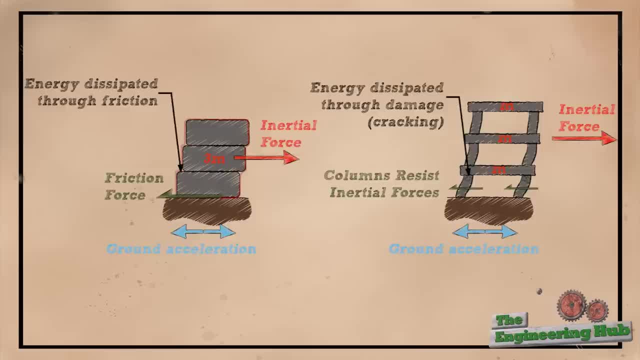 amount of force to be restrained. The restraining force in the block system on the left is the friction force, The friction force that keeps the blocks from sliding past one another. In regular buildings, the slabs compose the majority of the structural mass and are therefore associated with large 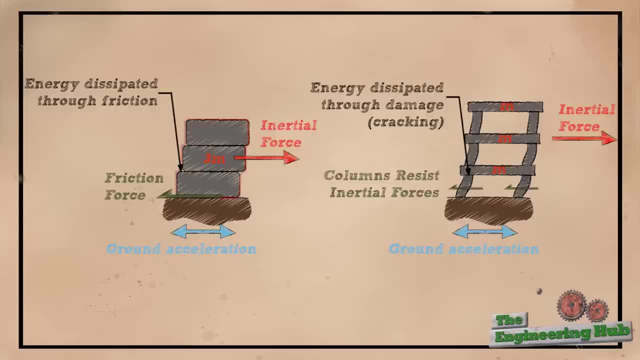 inertial forces. The force keeping the mass restrained comes from the structural members, such as columns, walls or bracings that try to oppose this motion, Since the structural members at the base have to resist the inertial force of the entire mass above them, usually the 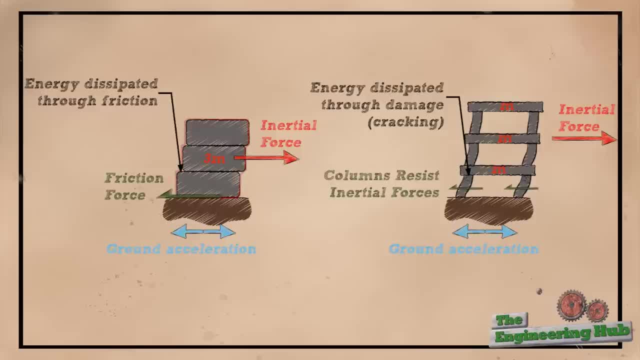 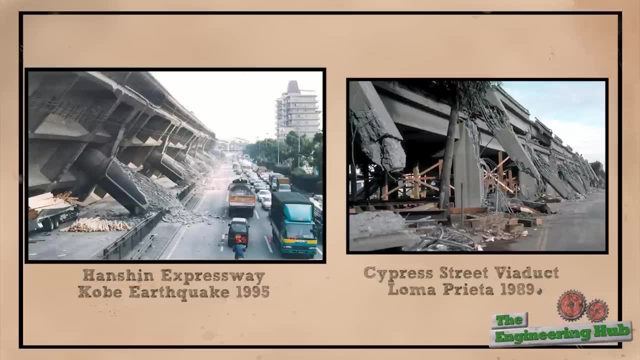 structural damage is concentrated around this area of the building. This damage can be seen on the picture on the left, which shows the damage caused to the Henshin Viaduct during the Kobe earthquake. In this case, the viaduct was too massive, producing huge base forces that the columns 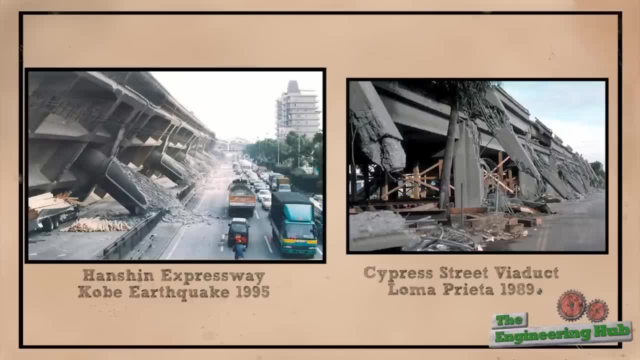 could not support. Similar scenario occurred with the Cypress Street Viaduct during the Loma Prieta earthquake. However, it is worth noting that fully restraining a structure against earthquake loads without sustaining damage is a very costly and impractical approach due to the enormous magnitude. 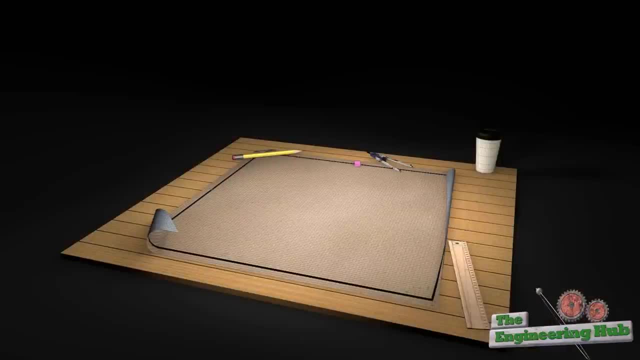 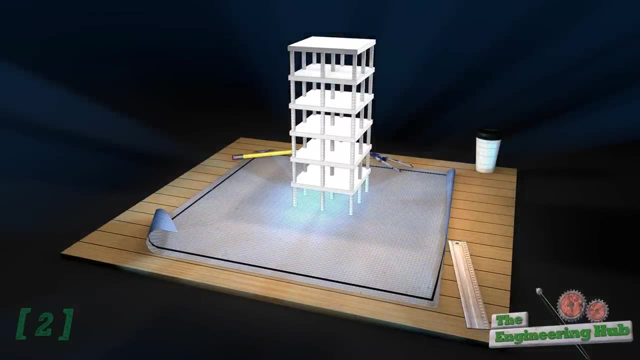 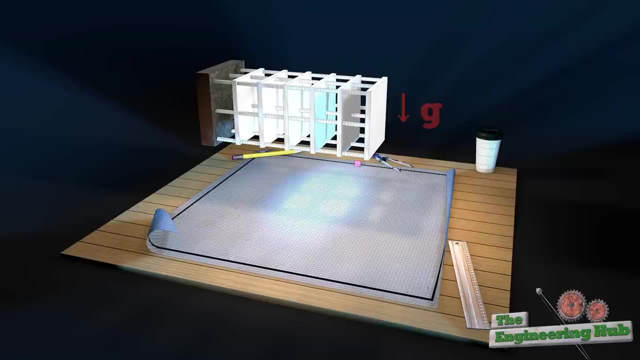 of these loads, The estimated peak ground acceleration for some places in California is as high as 1g. If the structure was perfectly rigid during an earthquake with a peak ground acceleration of 1g, the structure would undergo base forces as if it was built horizontally. 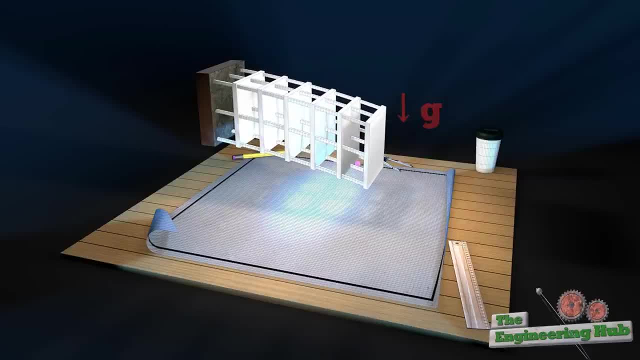 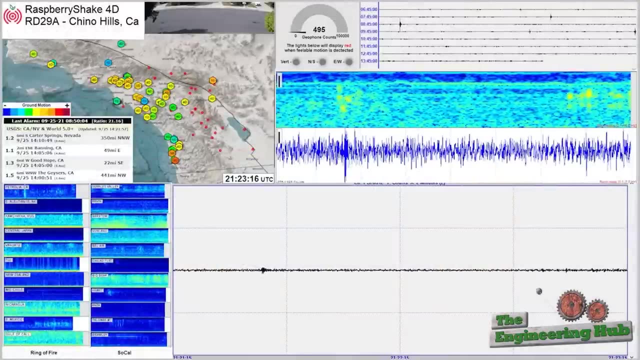 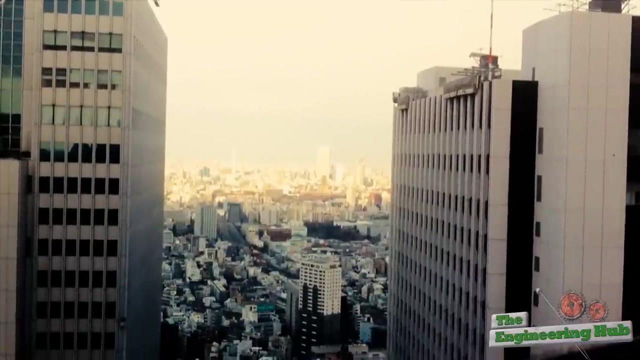 outwards from a cliff. Obviously, such structure is not feasible. No material can withstand such force. Because earthquakes shift direction rapidly, they do not sustain high accelerations for long periods. Therefore, structures that have long periods tend to be exposed to smaller loads. 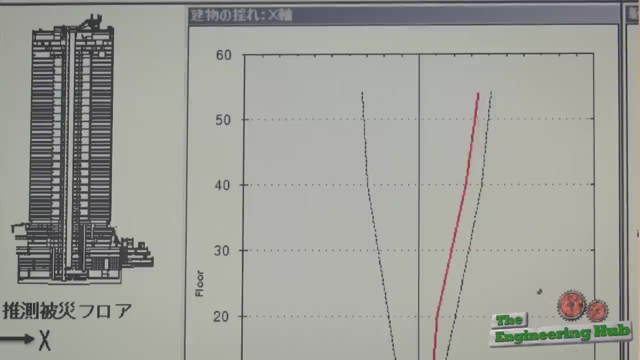 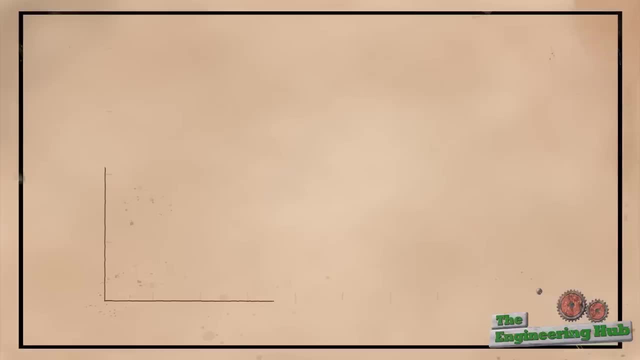 In other words, moving out of sync with the earthquake, would help the structure by cancelling out some of the motion. This can be seen on the so-called spectral acceleration plots. I won't go into detail how these plots are developed, but it is clear that for 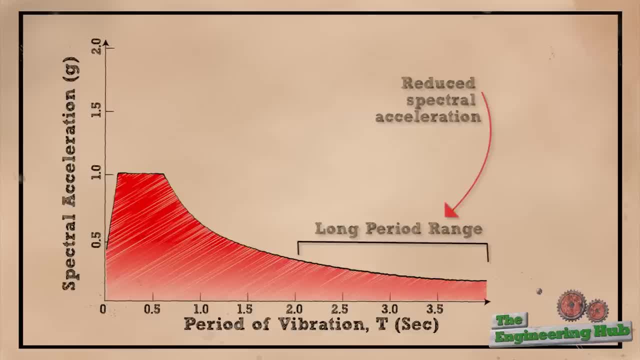 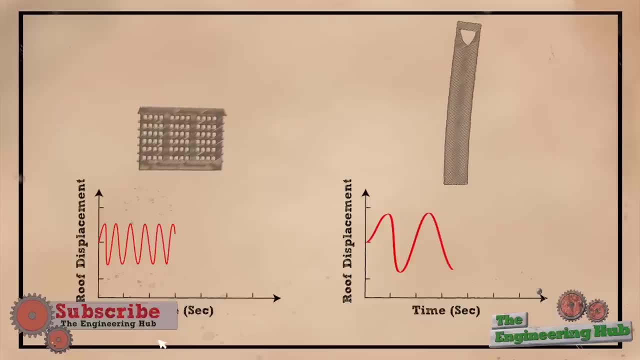 longer periods of vibration, the acceleration is significantly reduced. A period of vibration is the time that it takes the structure to complete one full oscillation. The period is dependent on the properties of the structure itself, mainly the mass and stiffness. The stiffness of a structure is heavily influenced by its height. This is 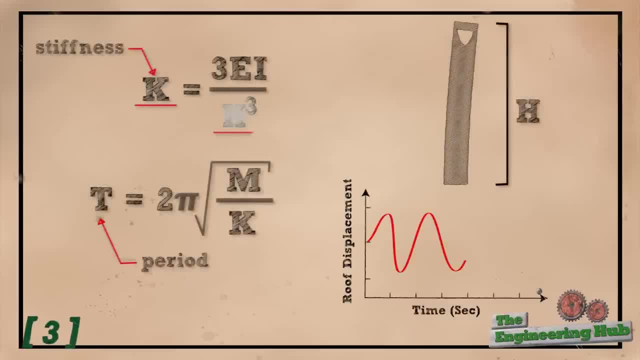 because the stiffness is inversely proportional to the cubic power of the height. Even though taller buildings are more massive, the structure is more stable. This is because the structure is more massive due to the extra material. their stiffness is exponentially reduced due to their 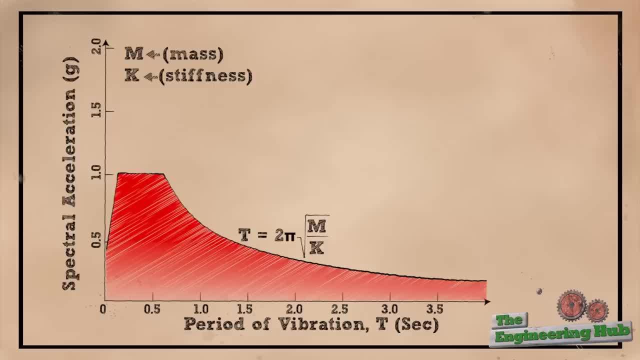 height. Therefore, taller structures end up in the long period range on the response spectrum. Since taller structures vibrate out of sync with earthquakes, contrary to popular belief, they perform better during an earthquake. But keep in mind, the response of a structure is also dependent on many other parameters that are not mentioned in 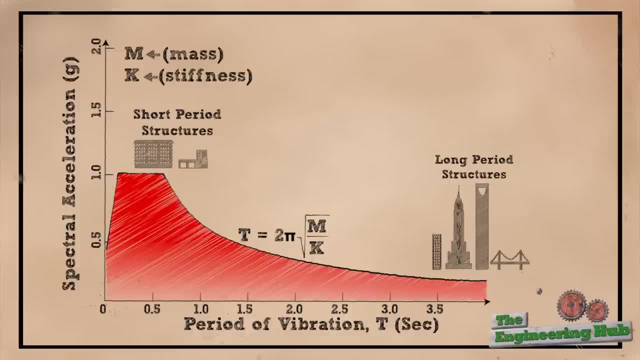 this video, such as the mass of the structure, For example. the mass of the structure depends on the size of the structure. This is why it is important to consider the mass of the structure. Soft soils could amplify the response of the structure.